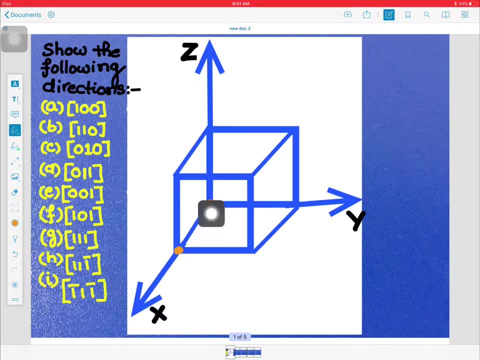 one unit in x direction. so we will reach here then. no, any propagation should be in y and z, because this is its origin in the 31st minute. so i'm already taken auff intention. that is one zero, zero to the one unit in x direction and i'll connect the on y and z to one y, one, zero and zero d two. 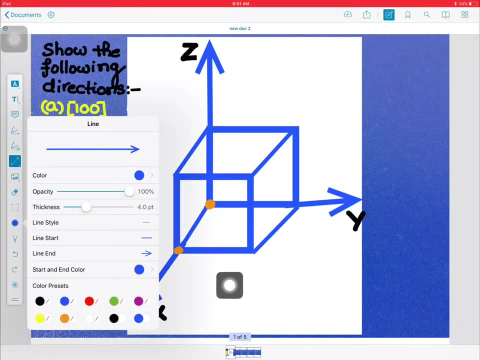 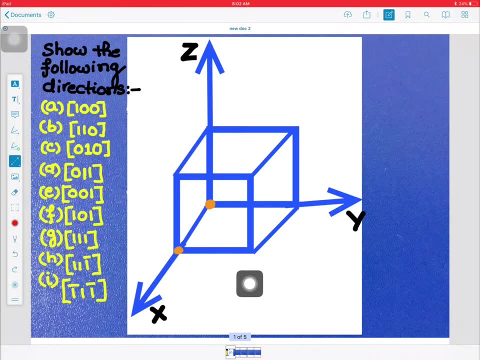 i'm trying to measure theesta possible intercept here. so only this: directions, so you can see these directions, this direction. okay, let me change the color direction. now let's see the next direction. that is 1, 1, 0. so in this case also, you have to first move to one unit in X direction, then one unit in Y. 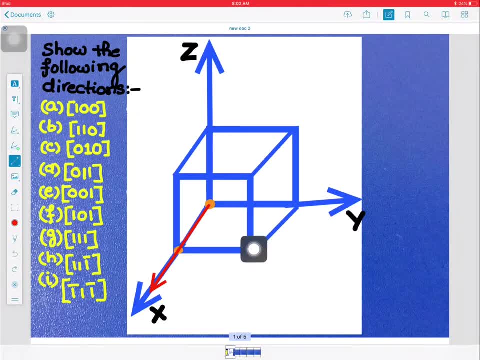 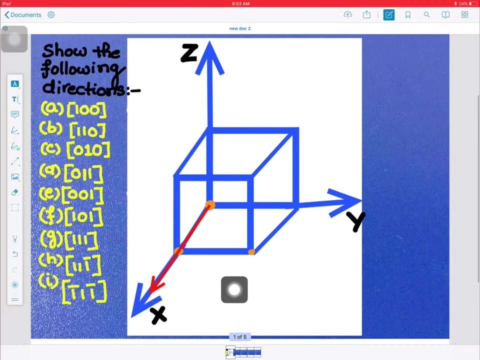 direction. so you will reach here. okay, you will reach at this position and there is no any movement or you know projection length in along the J direction. so this will be our final position. now you have to just meet them. so that will be. so you can see, this will be the, so that direction, basically this. 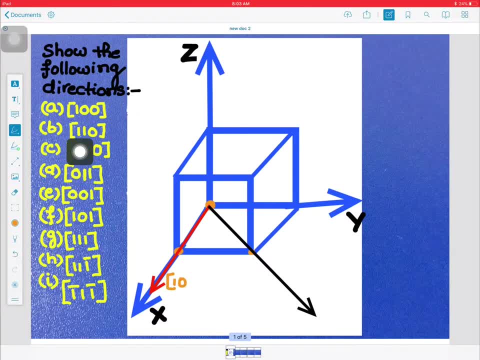 direction is one zero, zero. and this direction is what? one? one, zero. ok, now let's see the next one, the C, that is 0, 1, 0. so now we don't have to move along the x axis, because that is zero projection. now, Y axis, this is one. so we 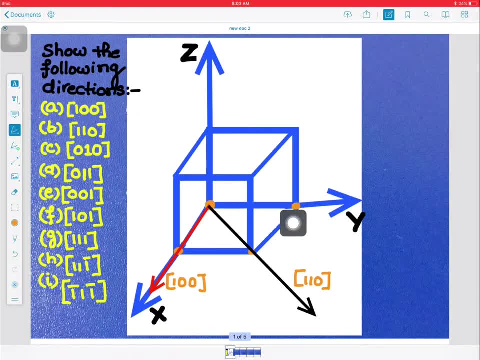 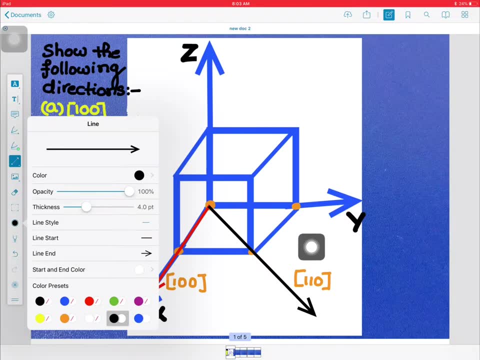 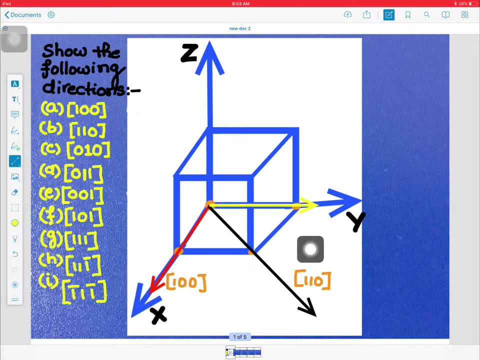 will reach at this position. one and Z axis: again zero. so now just we have to join this two lines and if we join, ok, this basically will be the. this will be our 0, 1, 0 directions. ok, next, the D1 is 0, 1, 1, so again, we don't have to. 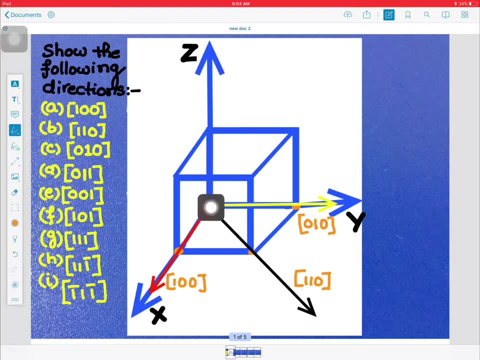 move along the x direction. so first we moved along the Y axis, so this is the first one unit. then along the z direction, so this is the first one unit and this is our final position. again, we have to meet this origin to this point. so again, what we have to do, 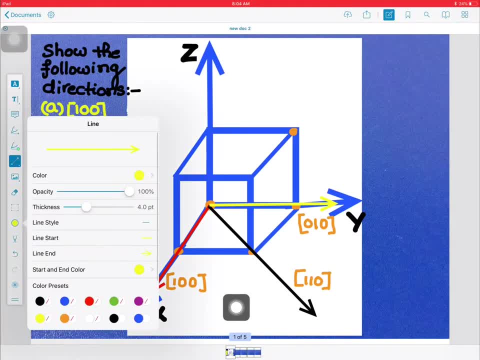 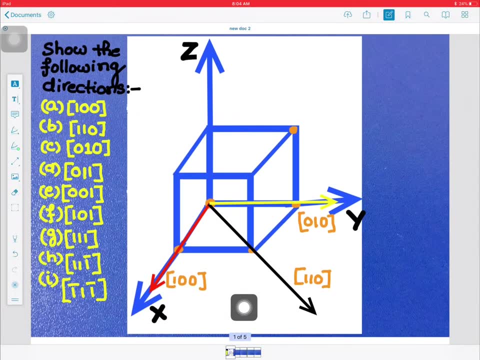 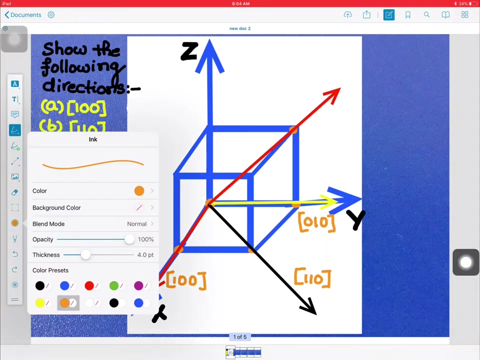 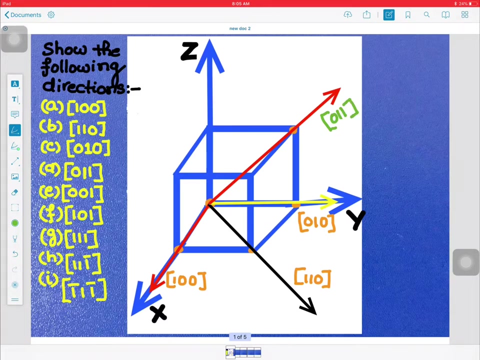 just meet it. okay, so let's. so this direction will be our d1, that is, the zero, and one that will be the zero one one. okay, now let's see, e is zero, zero one. so in that case we don't have to move along x and y axis, only we have to move along the z axis. so this is the one. 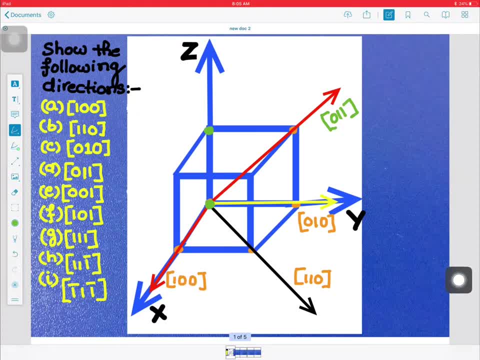 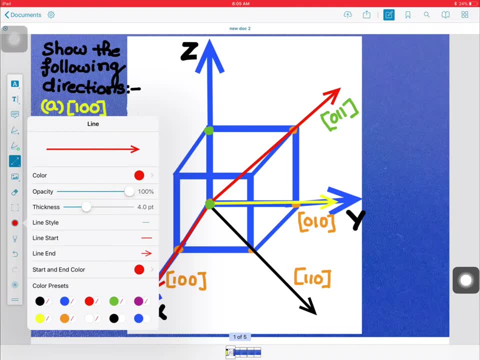 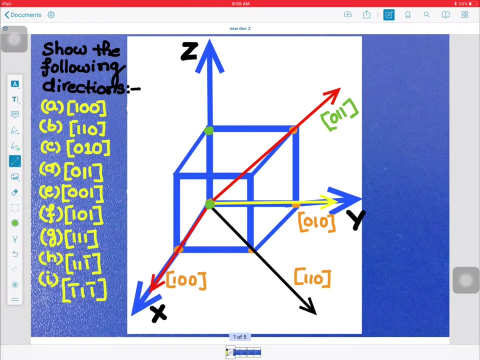 product unit. now we have to meet these two points. so join them. okay, just join it. uh, let's take this one, simply join them. so this will be third direction. basically will be: yeah, so this will be the zero one one. sorry, zero, zero one, zero, zero one. 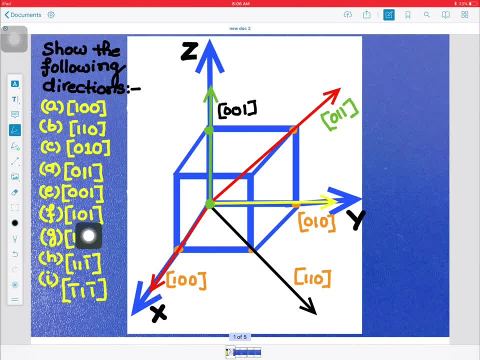 now, next f is one zero one. so first you have to go to one axis like the one, then along the y axis is zero. then you have to again move with one unit at z axis, so you will reach this position. so you have to meet these two points. so just make it, join them. 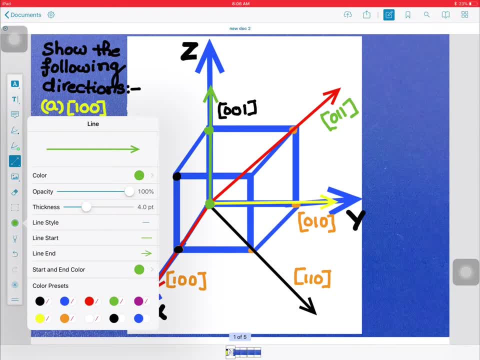 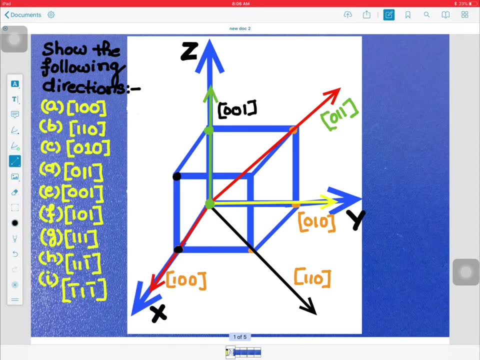 so just join them, i'm sorry, join with different color. okay, make it somewhat colorful, okay. so this direction, so this direction will be what in the f, that is, the. this direction will be one zero one. so one zero one. next is one, one and one. so let's see that. 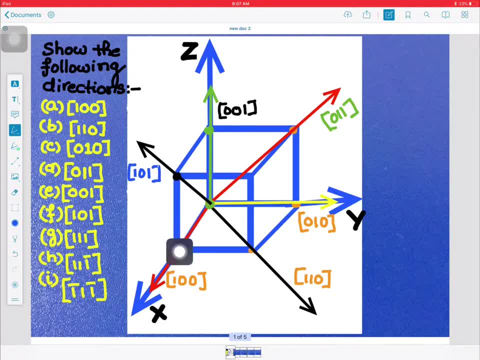 that you have to go to first one distance along x axis, so you will reach there. after that you have to go to along y axis at one unit, so you will reach here. then again with the z axis, so you will reach at this position. so yes, you have to join these two lines. so yes, 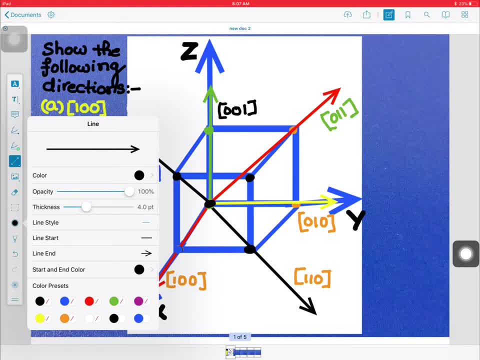 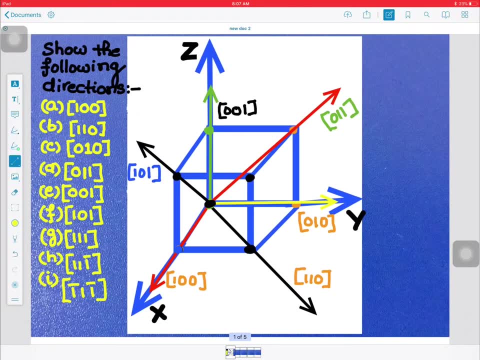 you can join them easily. join it, yeah, so this will be yes, so that will be our. the next one is what? one, one one. so that is the one, one, one direction. okay, next, what we have? one, one, one bar. one bar is negative, so in z axis it is negative, so you have to be careful in choosing the particular. 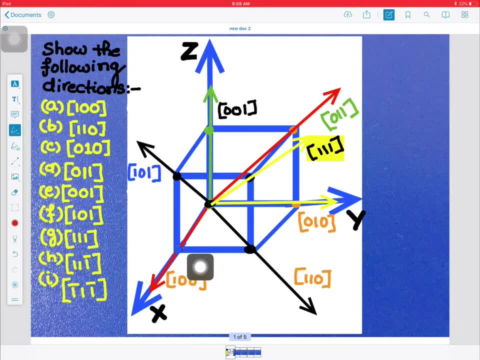 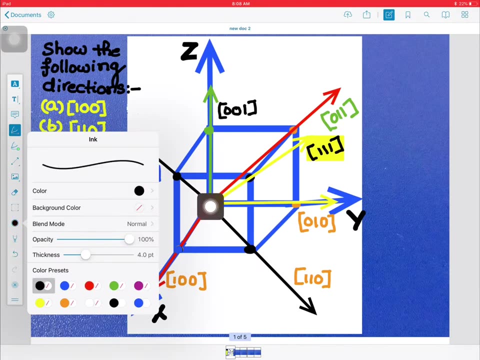 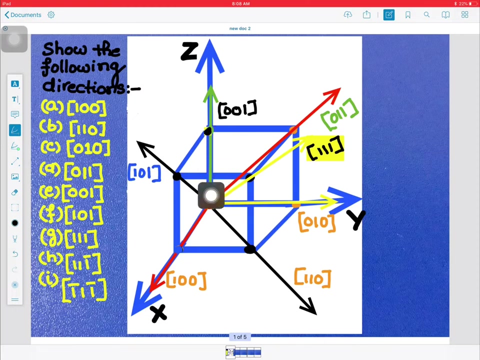 origin for this. if you choose this as the origin, you don't have z as negative, okay, you have only z positive. negative will be downward. so this is not, this will not be visible, okay, so let's see that, if you choose this one, so yes, z will be negative in downward direction. so this is the 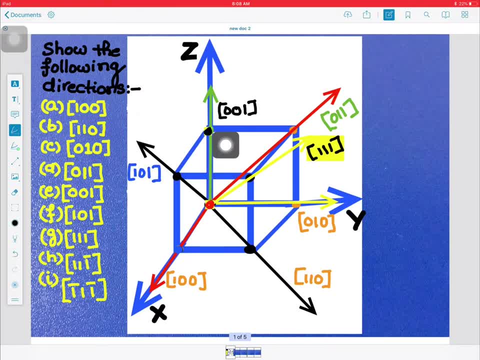 perfect origin for this. now, first you have to go to one distance along x axis, so this is x axis, so one. then you have to go along y axis, so then you will go to this place one, so one, one and one bar. then you have to go along the z axis, so that is the one bar. 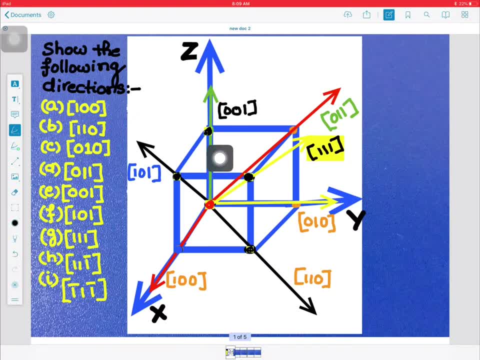 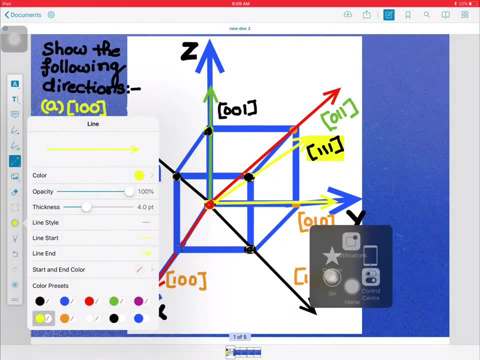 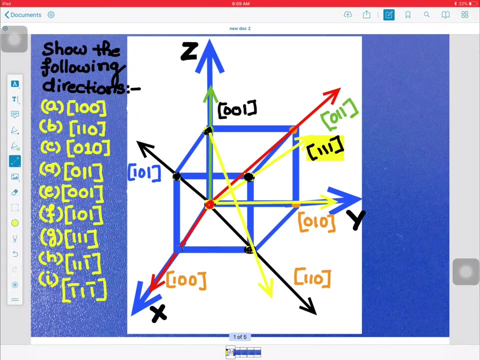 so, basically, this was our origin and this was our last position. you meet them together, use some different color, okay, use that, and just you have to meet them. okay, join them and this will be the word your direction. yeah, so that is the direction. that is one, one, one bar. one, one, one bar. 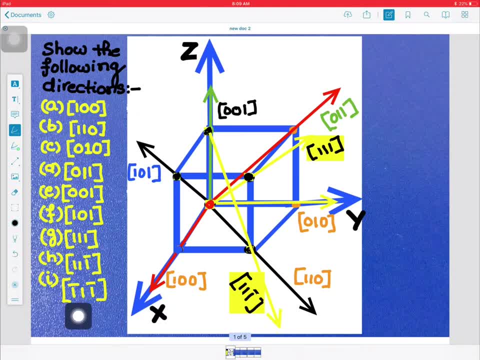 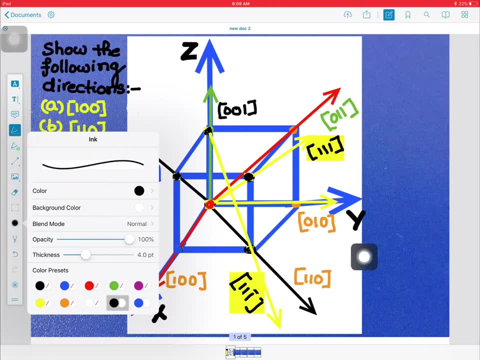 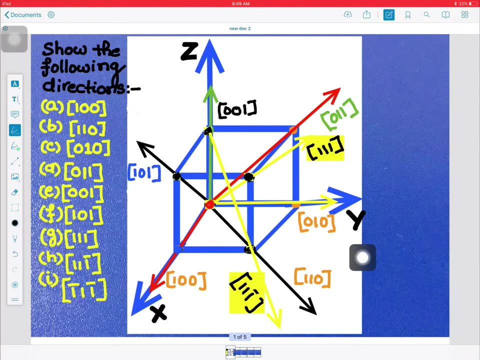 okay, next. next is one bar, one and one bar. so you have to choose a particular. you know you have to choose a particular crystallographic: that the origin in which there should be possible for the negative, for the x axis as well as z axis. so if you choose this position, it is not possible. if you 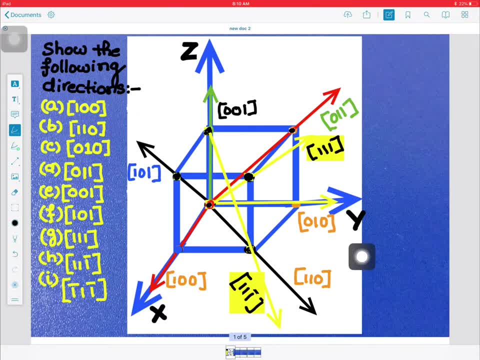 choose this position, so it will be negative for x axis, yes, negative for y axis, but, and negative of negative for y axis, yes, and negative for z axis, yes. okay so, but y should be in positive in this case, so you can't choose that one. if you choose this one, negative for x axis is possible, yes. 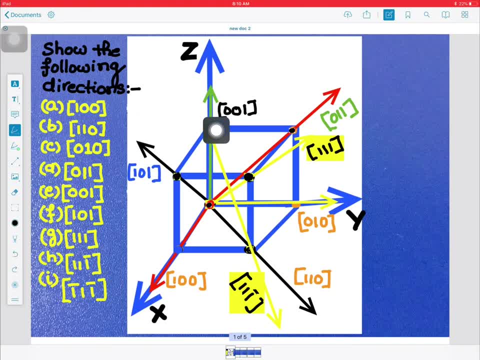 so negative for y axis and no, possible. but we don't know negative for y and negative for z possible. so again, this will be the origin. first we have to go to no. negative for x axis is not possible. sorry for this one. negative for x axis is possible, okay. y axis- we don't know negative okay and z axis. 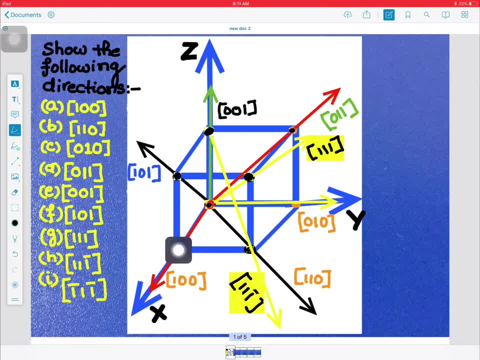 yes, negative is possible, so go for that. so this will be our origin in this case. so let's see, this is our origin, this is our origin in this case. we have to go minus one, so opposite of x, that is, we will reach here, then one, so we will.